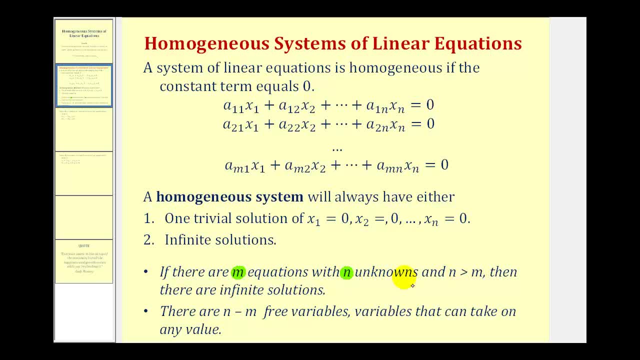 and n is greater than m- meaning the number of variables is greater than the number of equations- then there are infinite solutions And there will also be n minus m free variables. The number of variables minus the number of equations will tell us how many free variables we have. 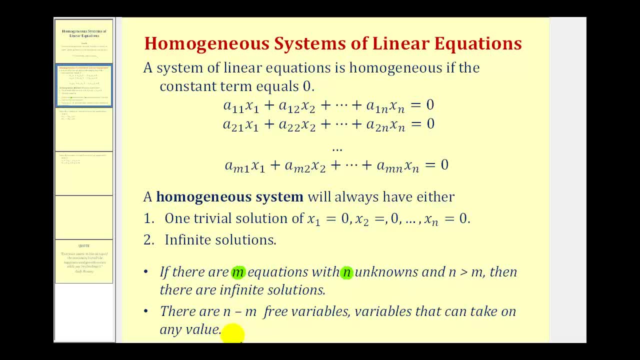 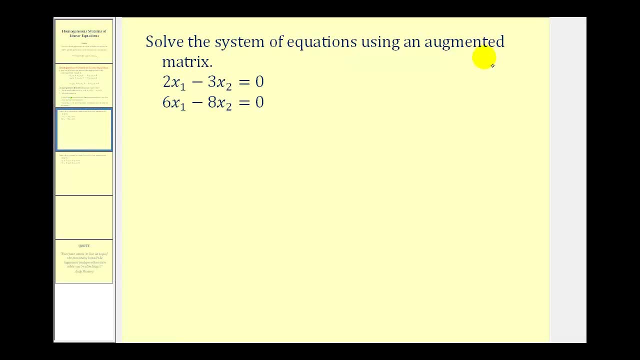 which are the variables that can take on any value, and we'll assign a parameter for them. Let's take a look at our examples. We want to solve the system of equations using an augmented matrix And notice how, because the constants are equal to zero, 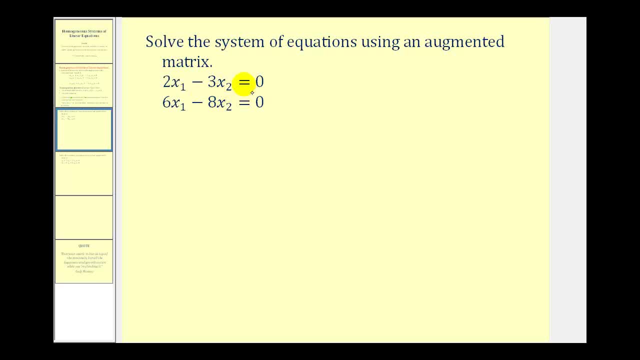 this is a homogeneous system of linear equations. Let's go ahead and set up the augmented matrix. So we have two negative three zero, And then we have six negative eight zero. We want to write this in row echelon form. 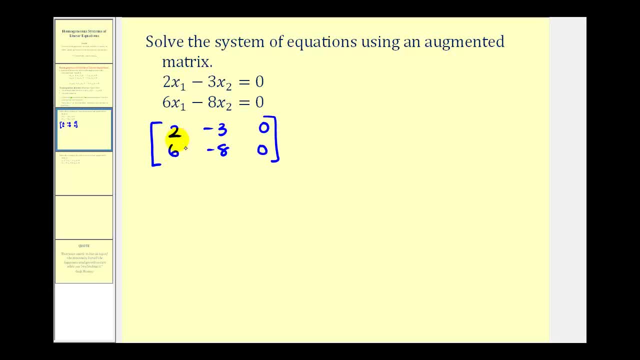 Let's focus on getting a zero here. Notice, if we multiply positive two by negative three, that'd give us a negative six. Then we could add that to row two. So we're going to replace row two with negative three times row one plus row two. 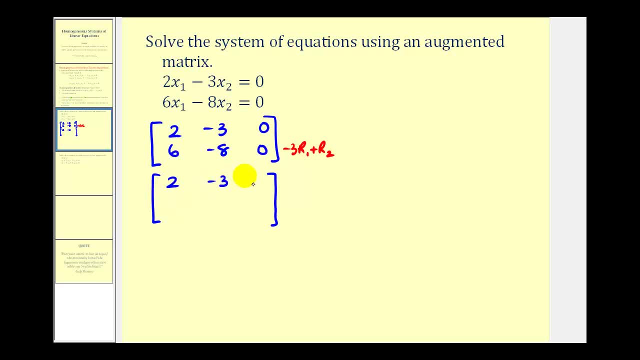 So the first row stays the same. Then we'll have negative three times two, that's negative. six plus six, that's zero. Negative three times negative. three is positive. nine plus negative. eight is positive one, and this is still zero. Going back up to our system, just for a moment, Notice how we have two variables and two. 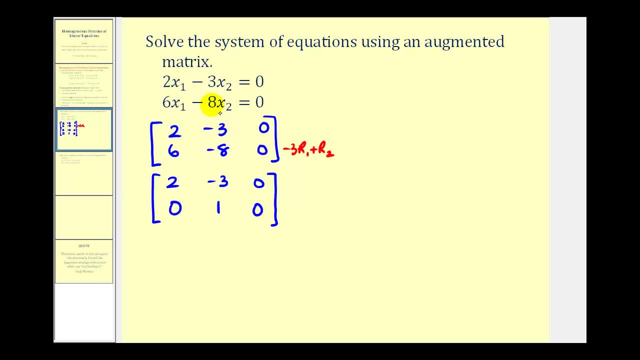 equations, which means for this system we have zero free variables. I think this is enough work to solve our system. Let's go ahead and rewrite this Now. we would have two x sub one minus three times x sub two equals zero, And also x sub two must equal zero. 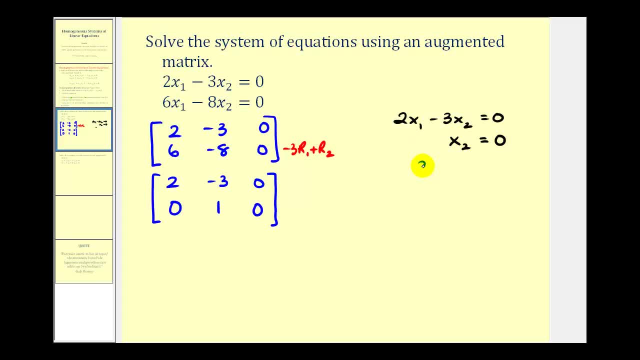 Well notice: if x sub two equals zero, the first equation becomes: two times x sub one equals zero, which means x sub one must equal zero. So, just as defined on the previous slide, a homogeneous system either has the trivial solution when the variables are equal to 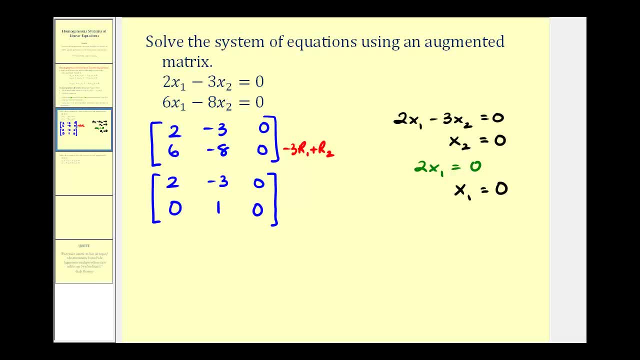 zero or has an infinite number of solutions. Here we have the trivial solution where x sub one equals zero and x sub two equals zero. Let's take a look at a second example. Notice, in this homogeneous system we have three variables and two equations, which means we'll have one free variable. 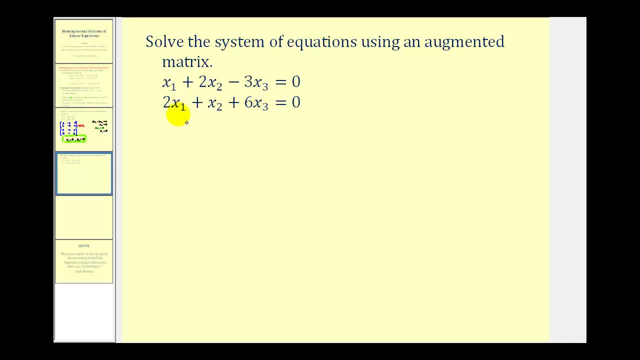 and an infinite number of solutions. So not only will we have the trivial solution when all the variables are equal to zero, we'll have an infinite number of solutions which we'll express parametrically. Let's first manipulate this system though using an augmented matrix. 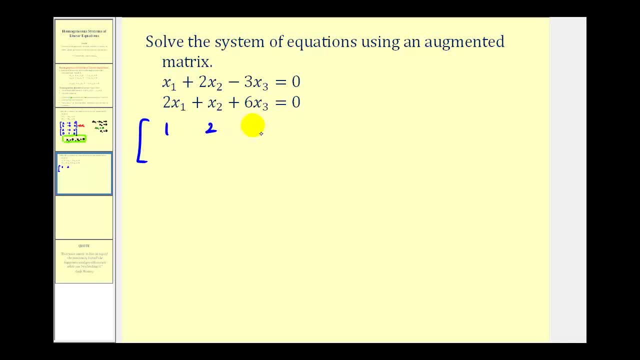 So we'll have one, two negative, three zero and two one, six zero. Let's start by obtaining a zero here. So we're going to replace this row with negative, two times row one plus row two, So the first row stays the same. 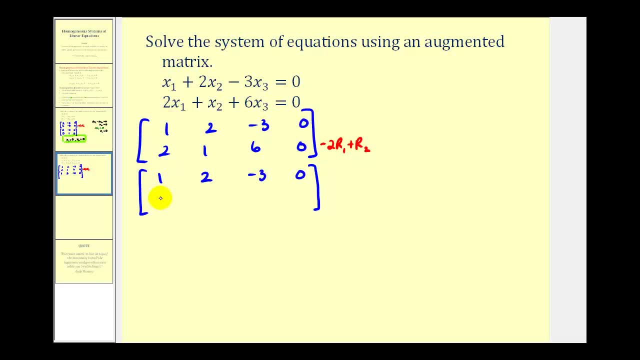 The second row is going to be negative two times one plus two, that's zero. Negative two times positive. two plus one, that's negative. three Negative two times negative. three plus six, that's six plus six or 12, we have zero. 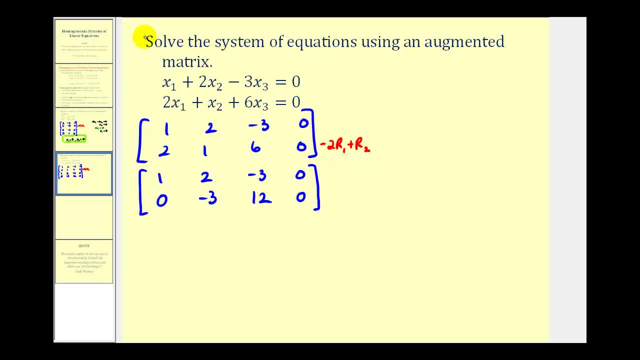 Now to obtain a one here, let's multiply row two by negative 1. 3rd First row stays the same. Second row would be zero one. so this would be negative four and zero. Now let's go ahead and rewrite this. 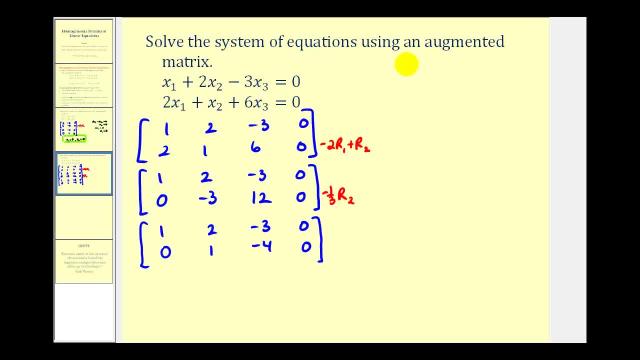 as a system of equations. Notice how the first equation didn't change. So we have x sub one plus two times x sub two minus three times x sub three equals zero. Second equation is now x sub two minus four. x sub three equals zero. 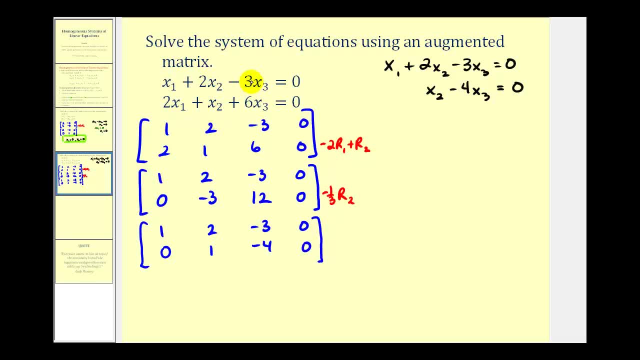 Again, because we have three variables and two equations. we have one free variable which we'll assign a parameter to. So let's let t equal some real number And then looking at our equations looks like it'll be easiest if we let x sub three equal t.